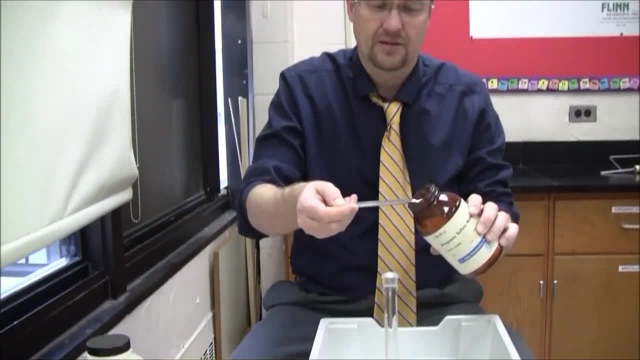 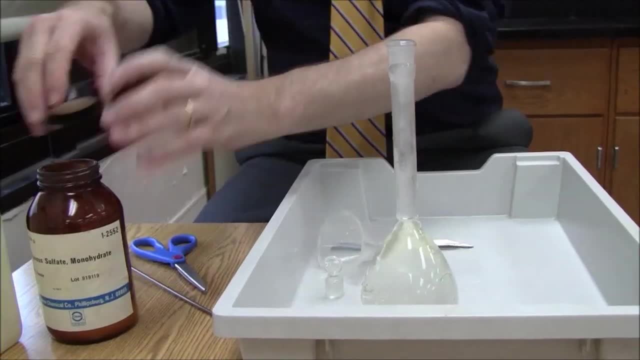 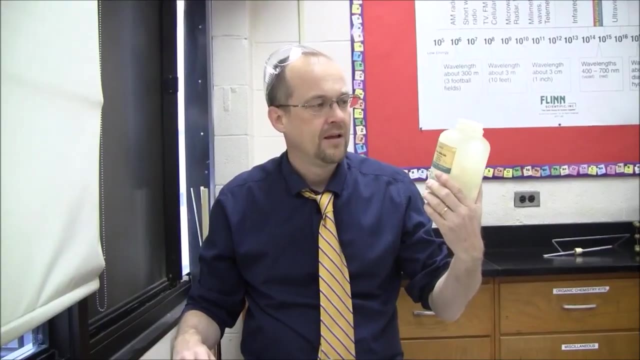 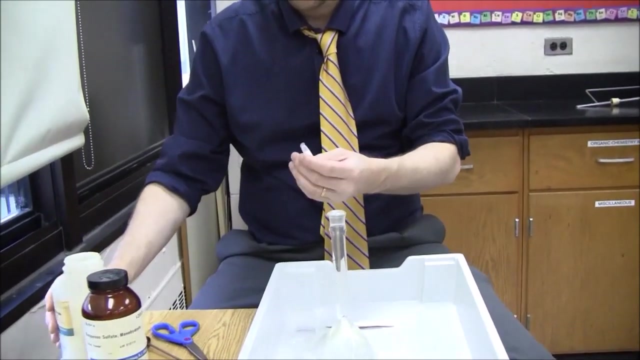 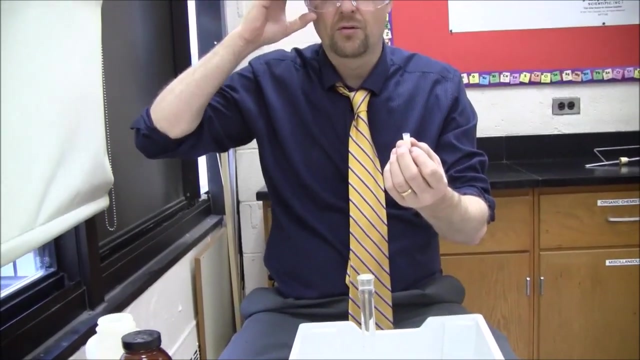 there we go smashing about that much. you put that in, okay, and strangely enough, one of these pillows an alkaline iodide azide pillow. so this supplies iodide and increases the pH because we need those hydroxide ions. cut that off, goggles on. okay, a bit of a second too late. let's try and pour. 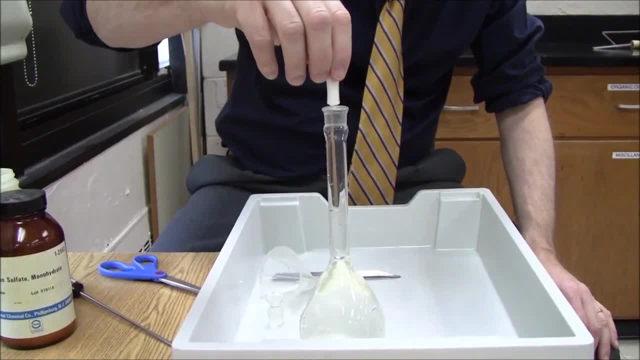 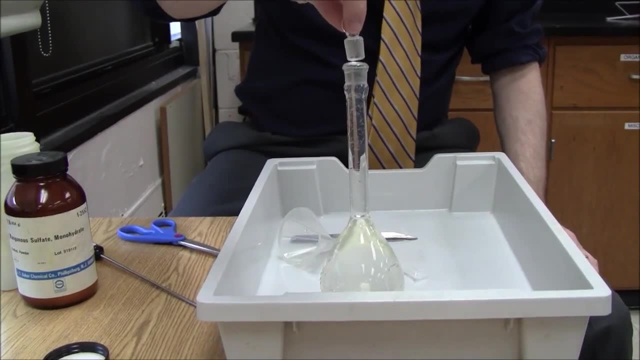 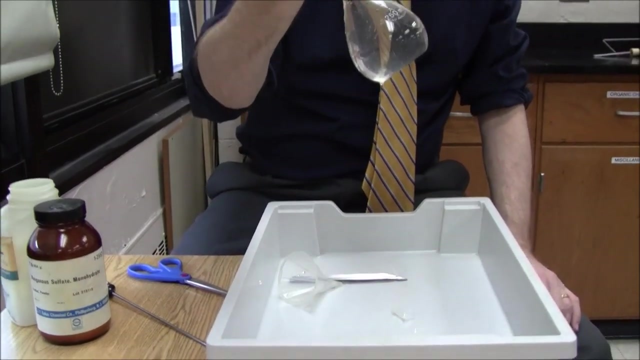 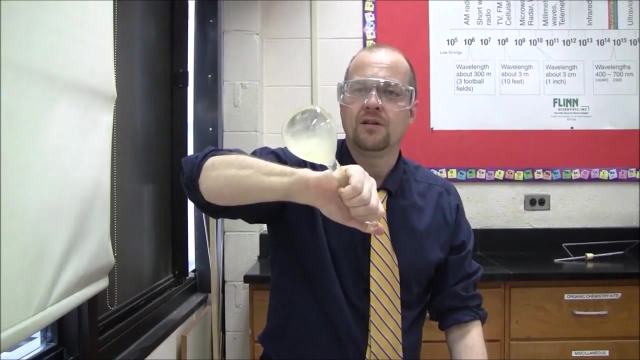 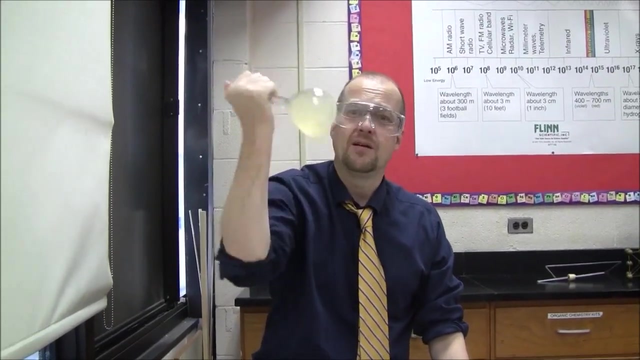 that in as well. that looks weird. cork it up, making sure there's no air bubbles, and shake it, baby. now if it turns brown, that means there is some dissolved oxygen and indeed it is turning brown. it's quite hard to shake it because if there's no air pocket to shake the liquid out of the water, 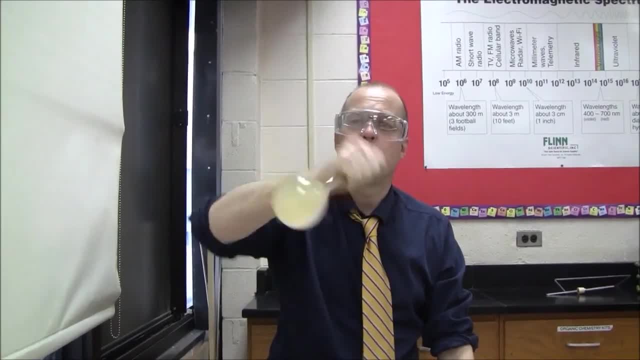 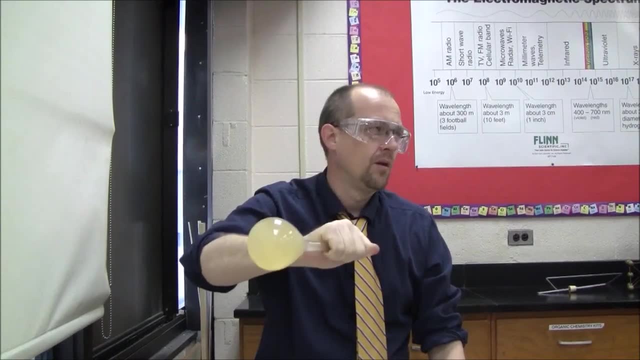 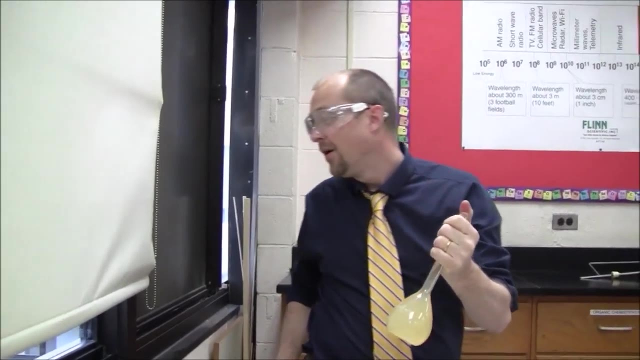 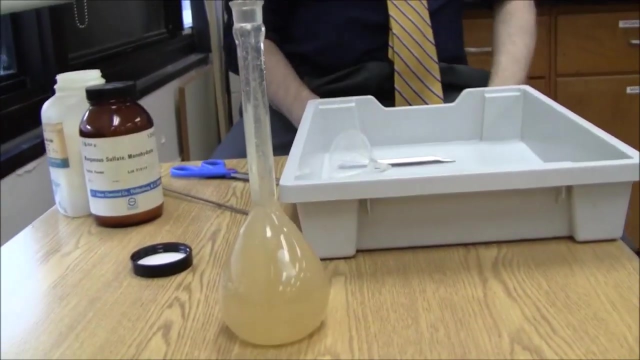 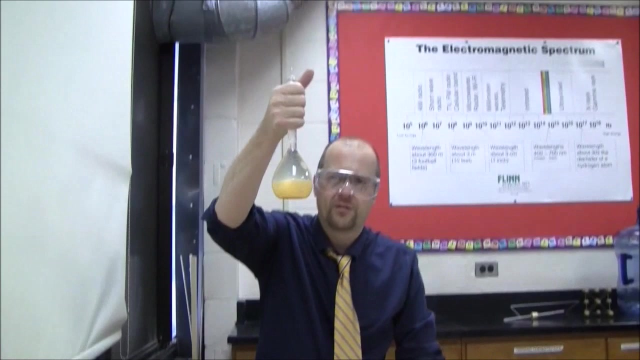 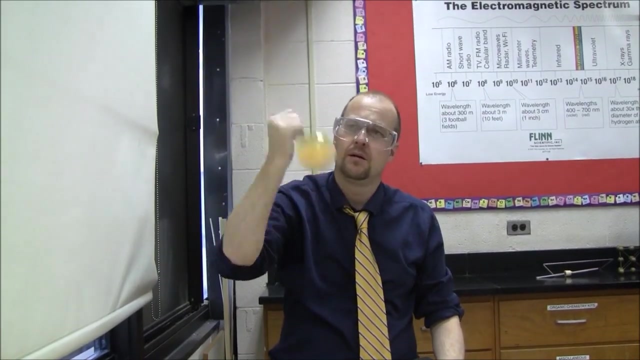 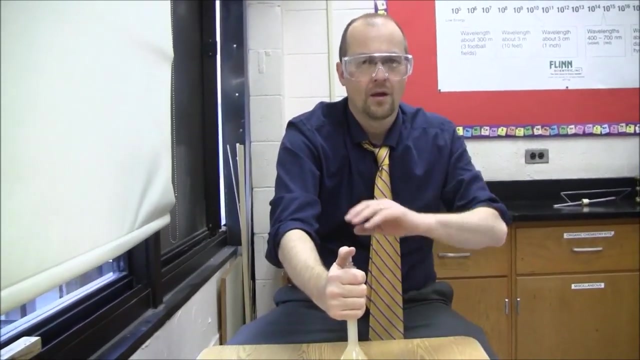 into the brown, is the manganese to turn into manganese. for set it down and you let the precipitate settle out about halfway and once the the flocculant or the precipitate has settled out about halfway, shake it up again and then wait again for the flocculant to settle. 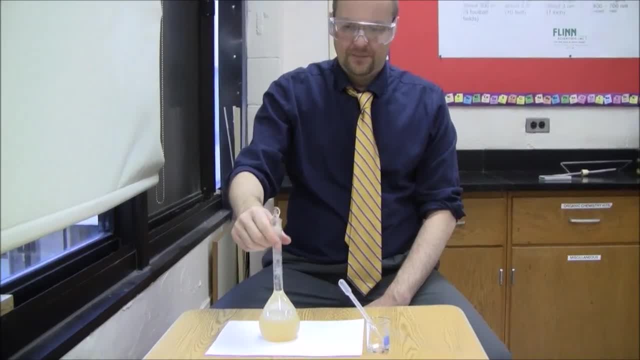 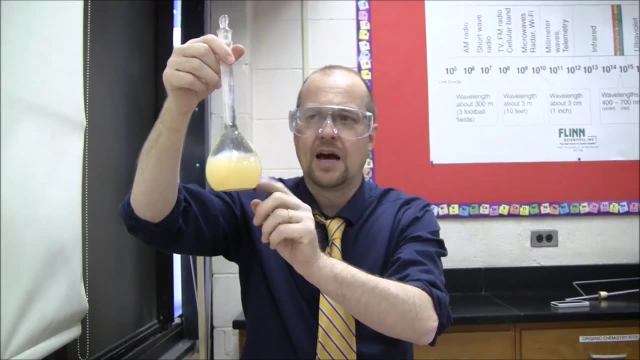 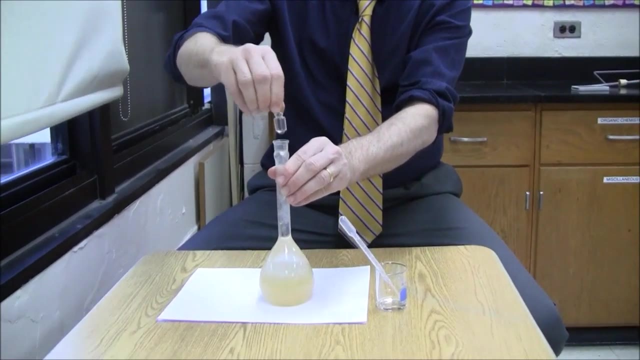 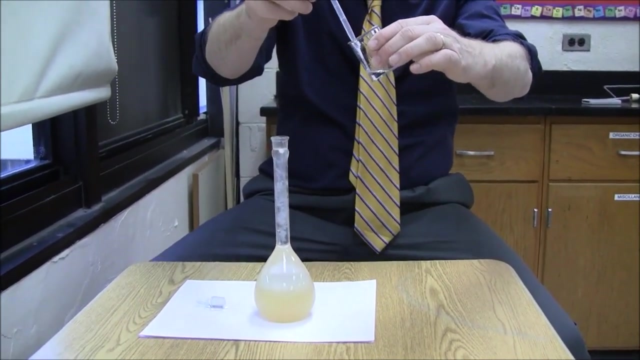 about halfway okay, so still no air bubbles, seems quite good. we had the manganese four ions here, which is kind of a brown manky color. now I have to reduce the pH for the next part, to work carefully, remove the stopper and I'm going to add two milliliters of concentrated sulfuric acid. move back a bit. 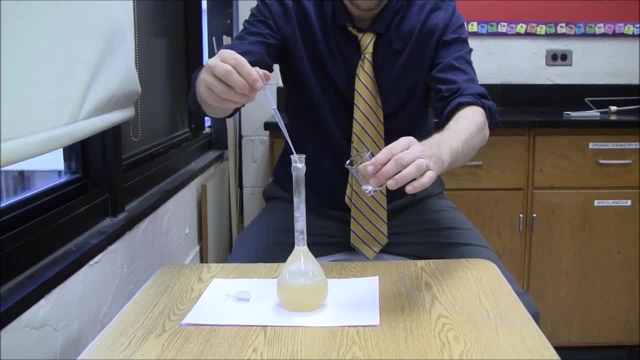 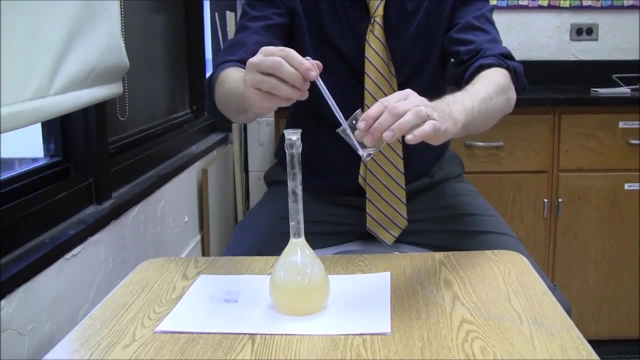 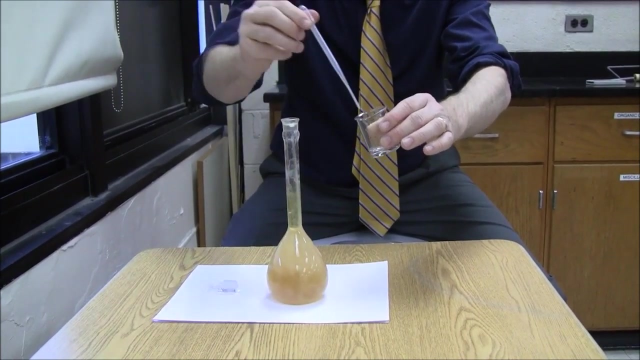 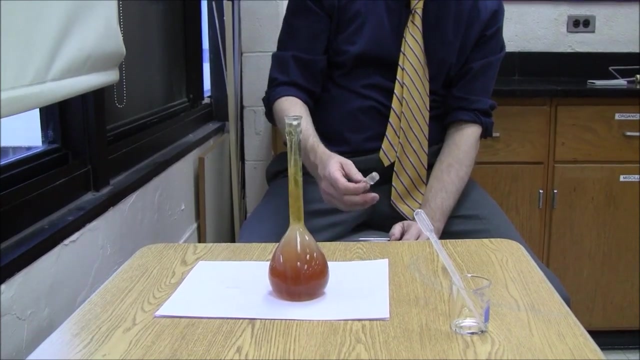 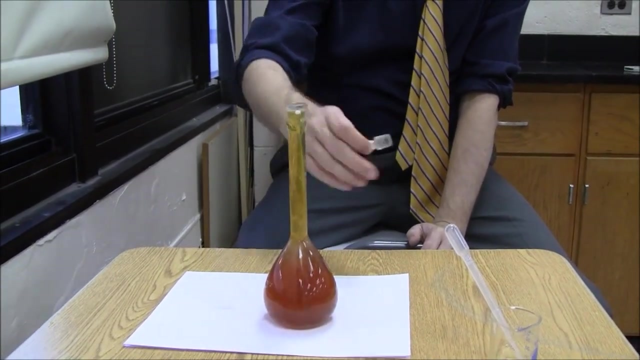 in case I spill it. that was just under two, so this is an excess. doesn't have to be exact, all righty, and you can see the reaction taking place here. the new brown color is iodine molecules being formed all the way through and the kind of cloudy manganese four has turned into manganese. 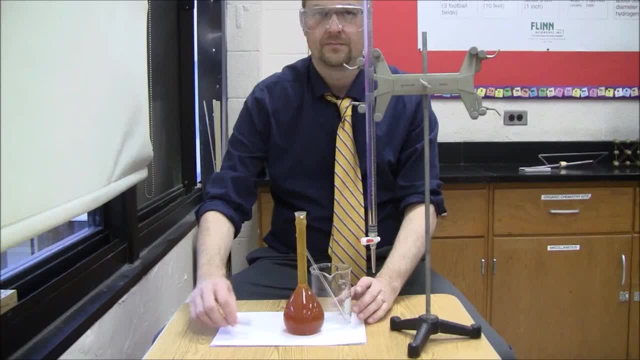 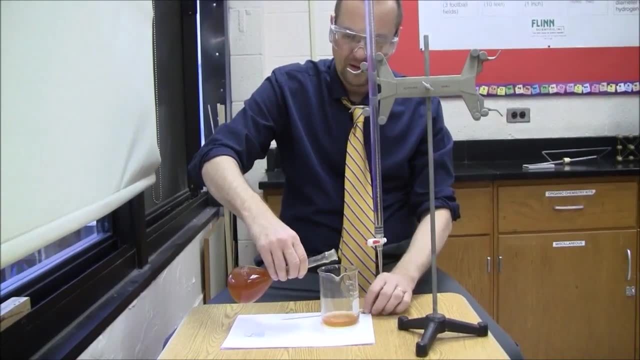 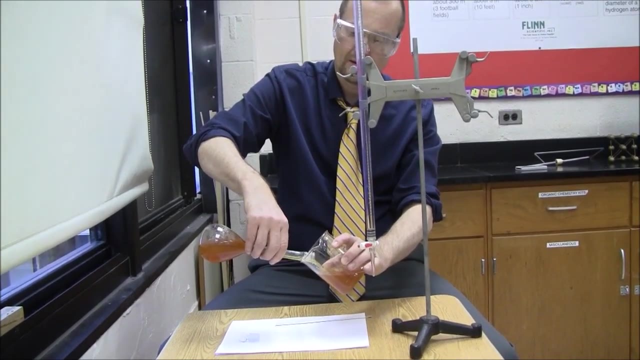 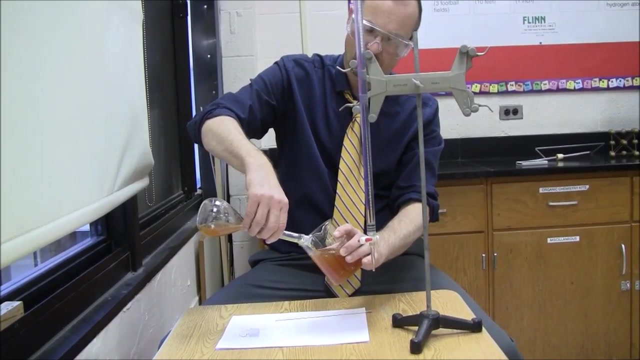 two. okay, now transfer your solution, because we can't really do a titration. oh and you know what? it's pretty stable, but you don't want to aerate it any more than you have to, although the number shouldn't change, because these chemicals you've added to stabilize the oxygen level and no reason. 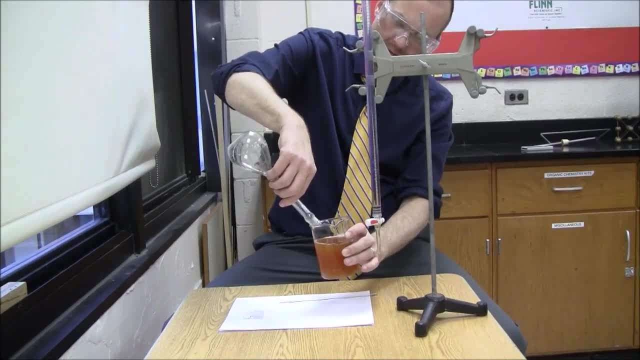 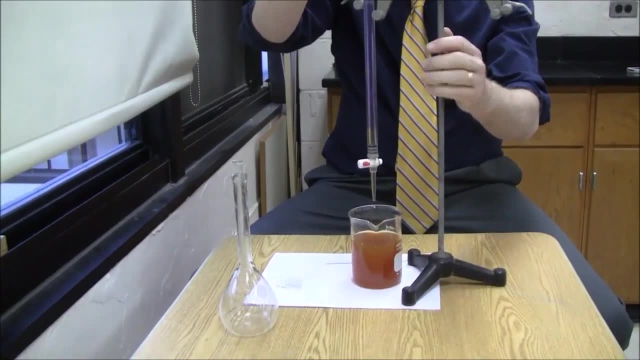 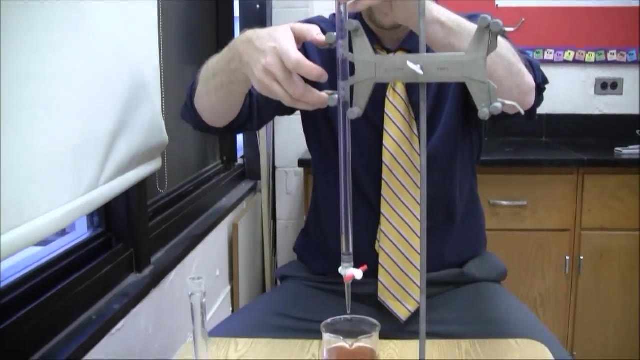 to tempt fate. all right, now we're going to do a titration. this is sodium thiosulfate. now, if I wasn't so brave, I'd split this sample in two to give me two tries at doing it. but let's see if I can titrate first time. 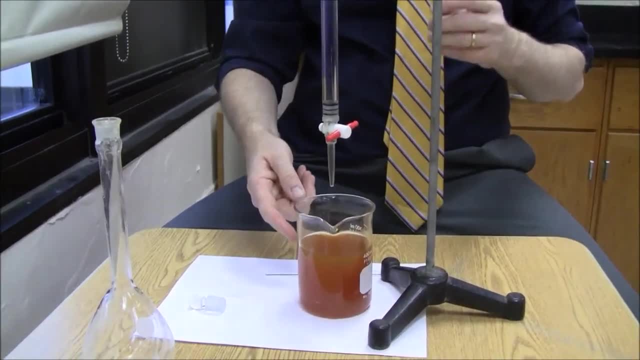 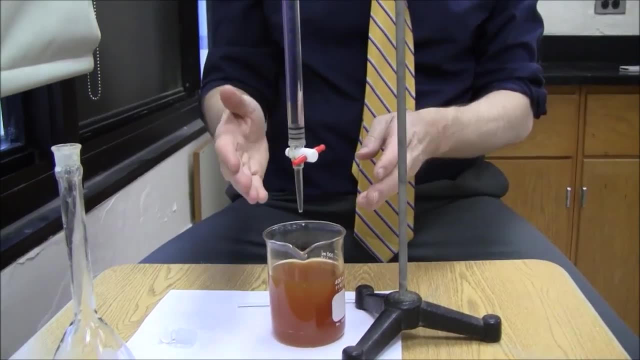 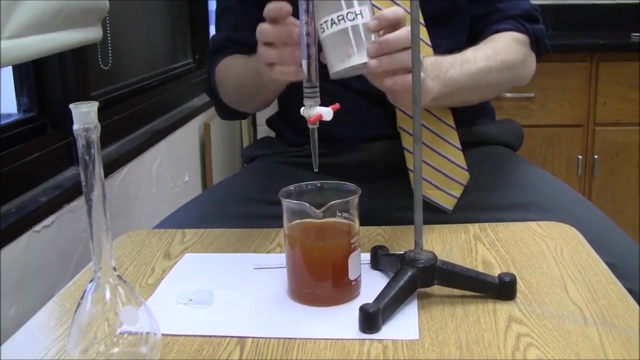 sodium thiosulfate is going to turn the brown by two iodine molecules into colorless iodide molecules. the transition from brown to not brown isn't as obvious as you'd like, so when I get close to the end I'm going to add a little starch and that's going to sharpen the. 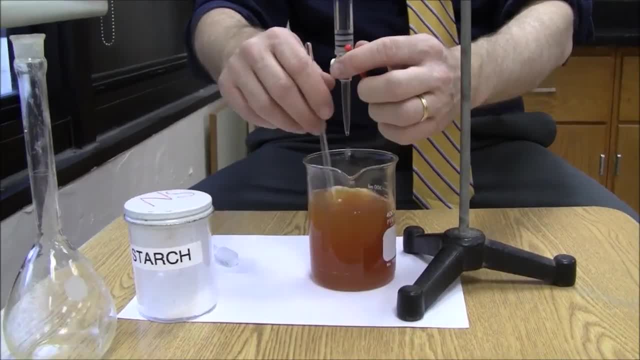 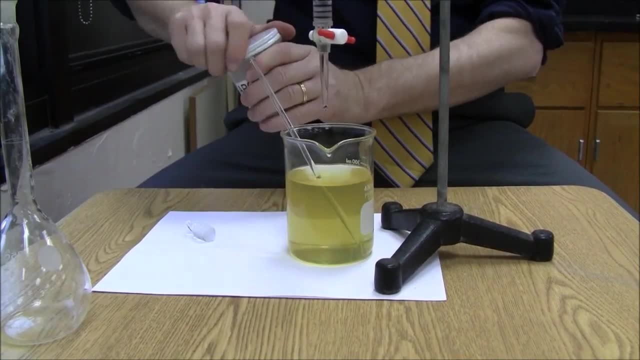 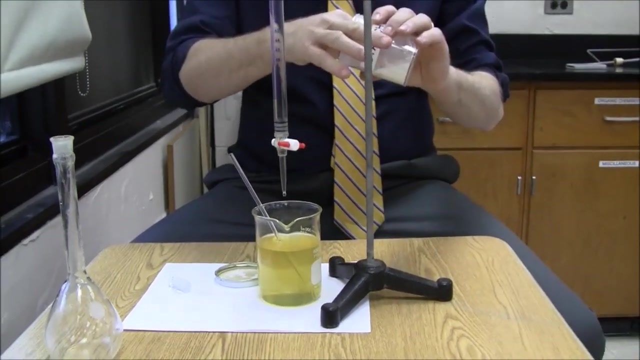 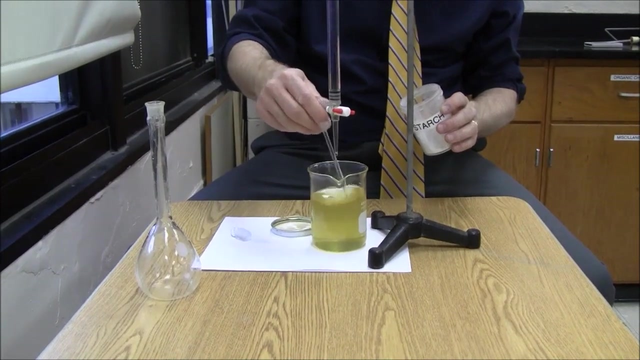 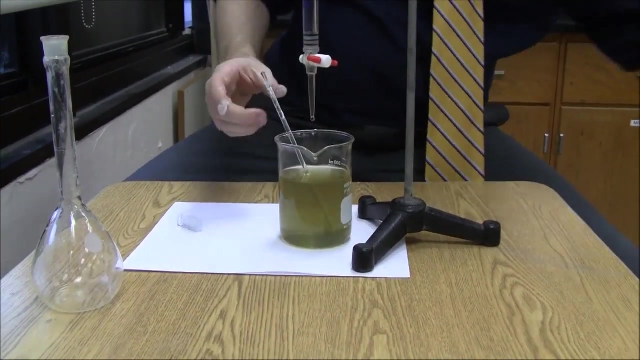 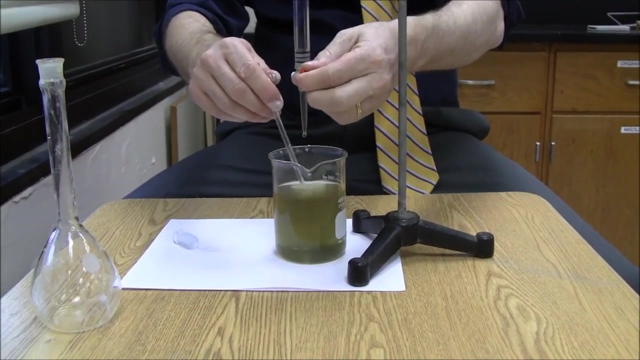 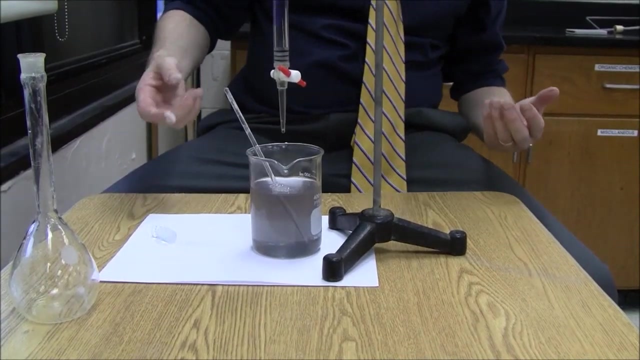 end point: add a little starch, non-toxic. literally a pinch, literally two pinches. okay, so the end point is now sharpened. it's hopefully going to be one drop changes everything. now that might be the end. I can't tell, so I'm going to take a reading. it's exactly. 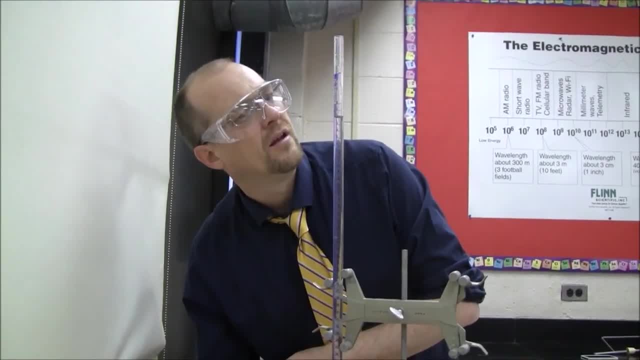 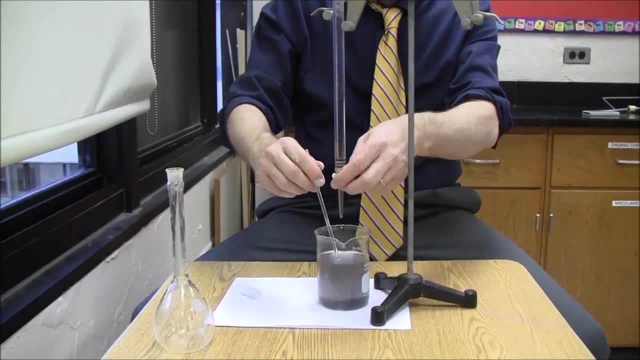 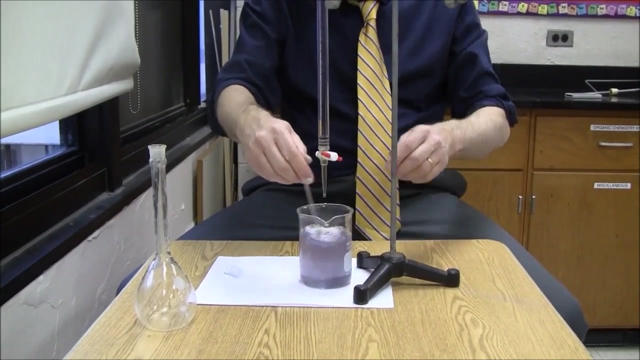 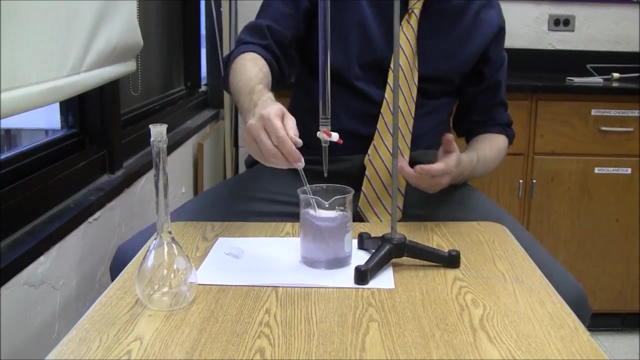 1.95 milliliters. that's the end, so I'm gonna remember 1.95 milliliters, or you probably should write it down if you're doing the experiment now. let's carry on and see if this is indeed the end. seems to be getting more colorless. let's see if. 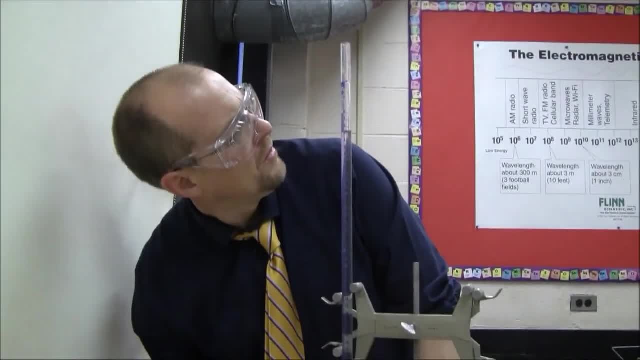 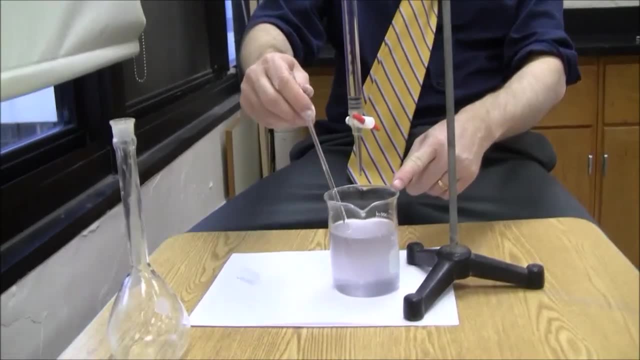 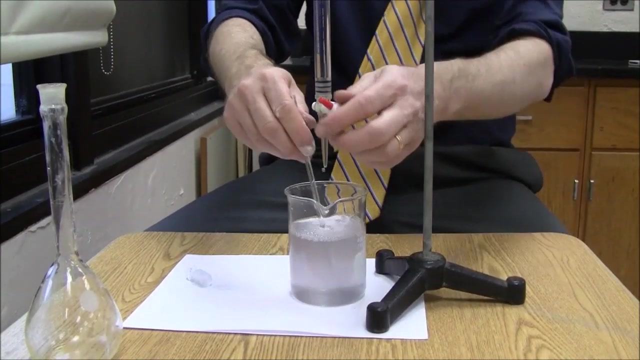 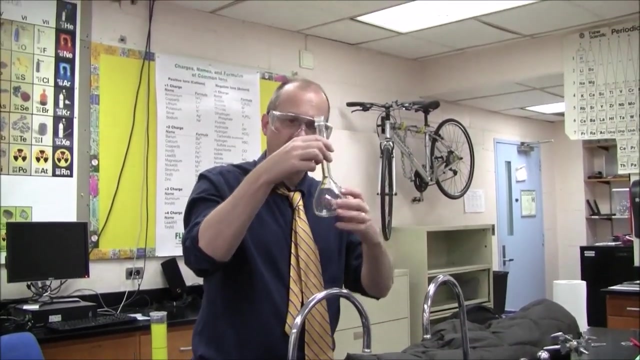 that's the end I'm writing down in my brain: two point two point seven milliliters. two point seven milliliters, up. you know what, it wasn't an instantaneous reaction. I think we're pretty much down at two point seven, so I need to know the total volume of this. I know it says 250, but it's only 250 up to. 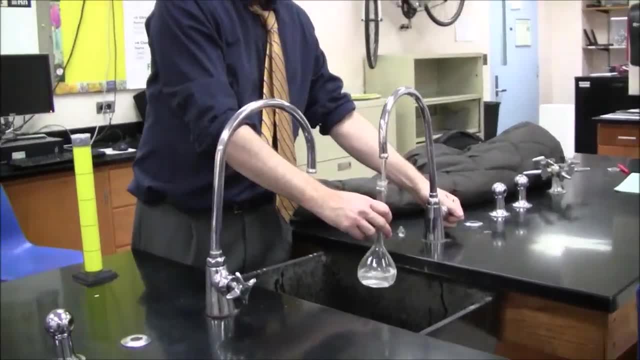 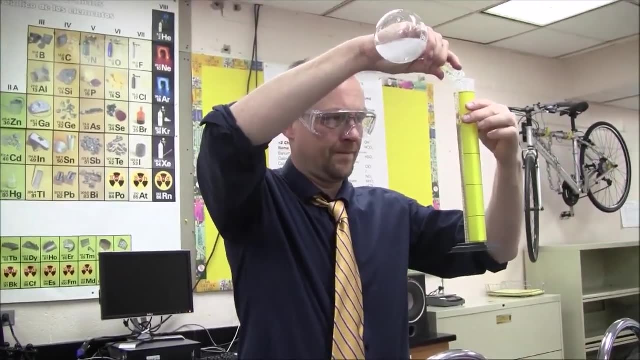 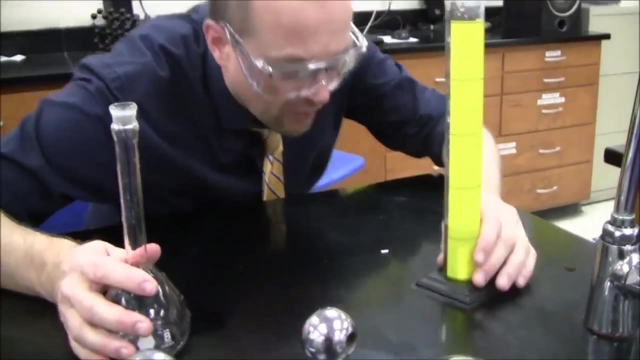 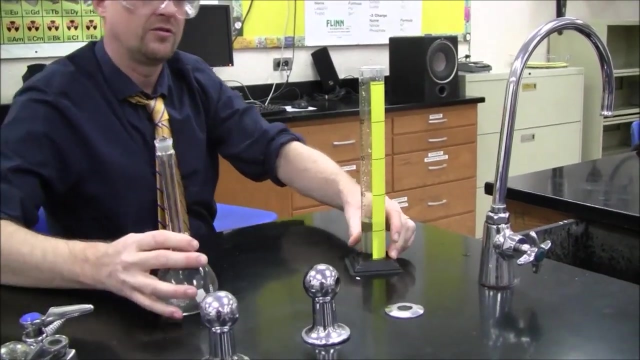 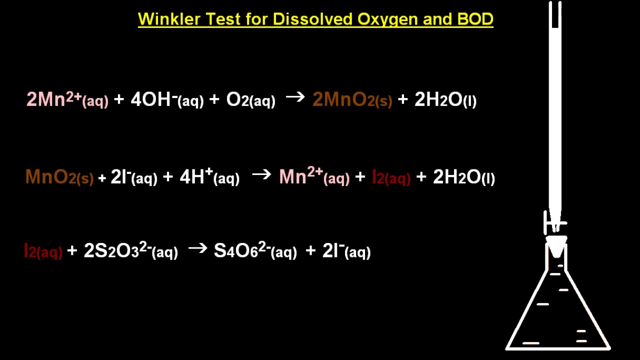 that line. there's a little bit more, so put it down to measure the meniscus like we're taught to in high school: 262 milliliters in total. this was okay. so these are the three equations. you won't be asked to remember them, but you'd be asked to use them. 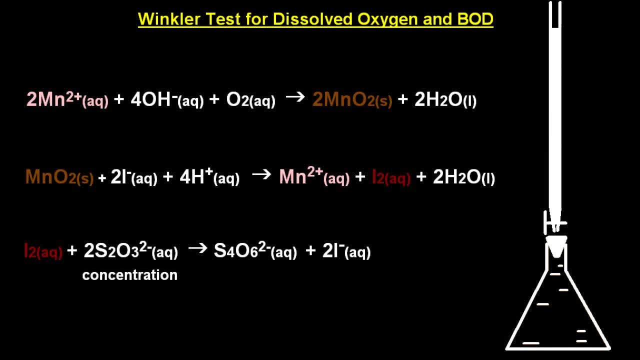 so that's the end of the experiment. Thank you for watching. So if I know the concentration of the sodium thiosulfate and I know the volume of sodium thiosulfate I've used in my burette, I know the moles. if I know the 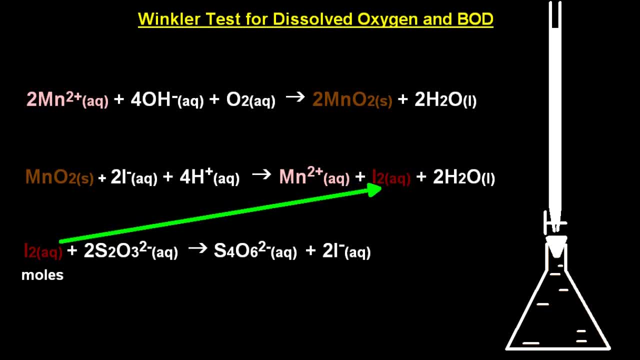 moles. I can work out the moles of iodine, which is the same as the moles of iodine there. and if I know the moles of iodine there, I can work out the moles of manganese 4 oxide, which will be the same as the moles of manganese 4 oxide there. 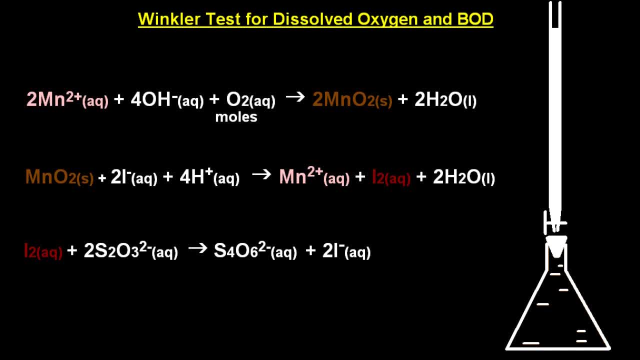 I once. I know that I can use that to work out the dissolved oxygen content. Now, if I know the moles of dissolved oxygen and I know the volume of water that I used, I can work out the concentration. and so that's a broad overview of the theory. 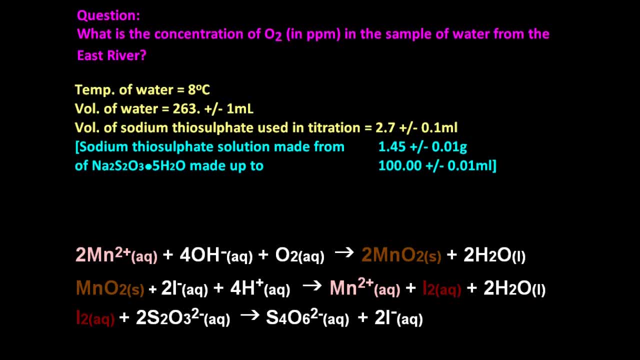 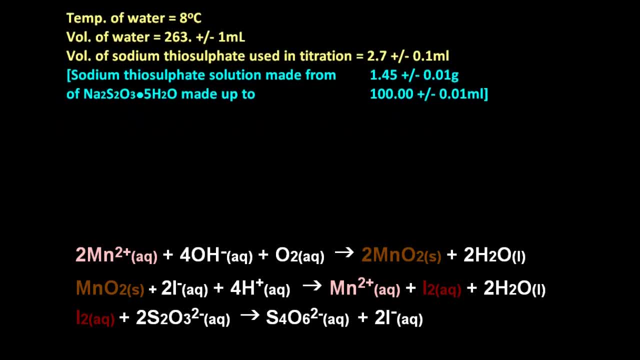 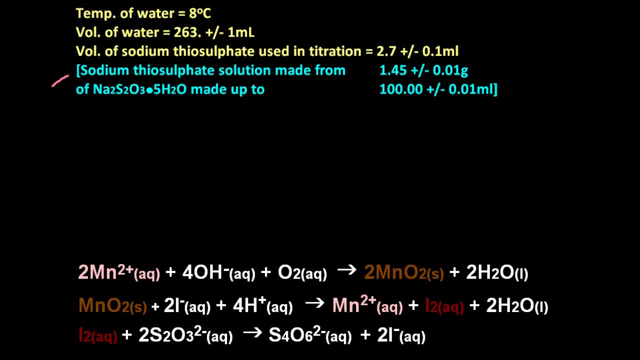 Okay, so the moles of thiosulfate first of all. just tidy up a bit. So, looking at the solution of sodium thiosulfate that was in a burette, let me work out the concentration of that. So that's moles over volume and moles is mass over molar. 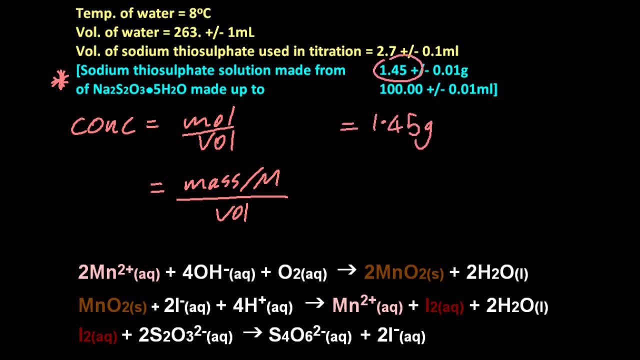 mass. So putting in the numbers molar mass from the bottle and the volume in decimetres cubed, that means the concentration of sodium thiosulfate in my burette, is that Now I'm using one more sig fig than I need. there's two sig. 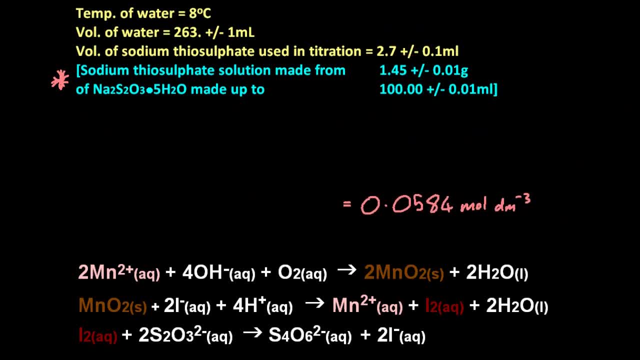 figs in the 2.7. so I'm gonna save three sig figs and then work it all out later. Okay, Now I know the concentration of sodium thiosulfate in the burette and I know the volume. I can work out the moles. So concentration is moles over volume, which? 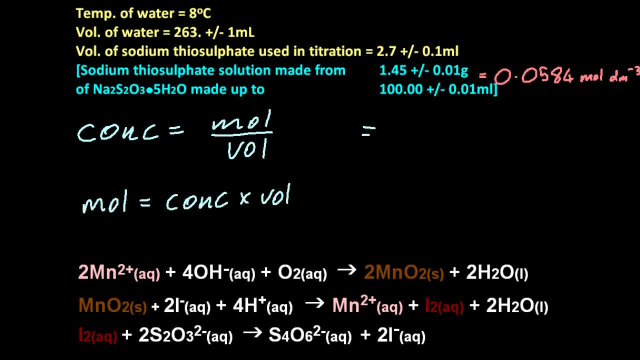 gives me moles is concentration times, volume Concentration- I just worked it out. and the volume, well, don't forget to convert to decimetres. cubed by dividing by a thousand. Okay, that's how many moles of thiosulfate in the burette. 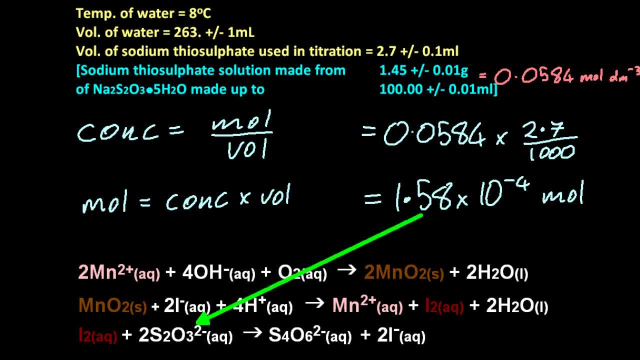 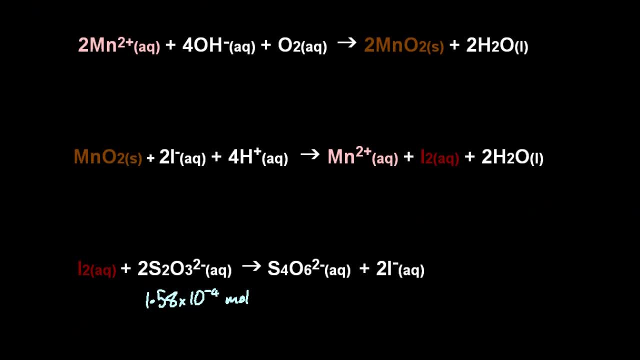 So that's the moles of thiosulfate I have. So that's the moles of thiosulfate, and since the ratio is one to two, I must have half of that moles of iodine. That number now moves up to the middle equation, And I 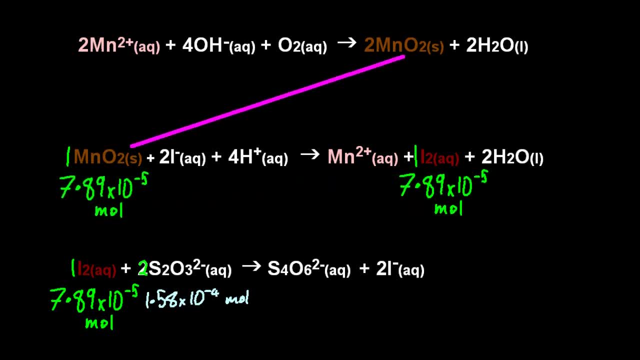 wanted to know about the manganese. for oxide it's a one to one ratio. it's the same number of moles. move that number up, don't double it. it's tempting to double it, but just leave it as it is. Now the oxygen is going to be half the number of moles. again looking at the ratio- smash. 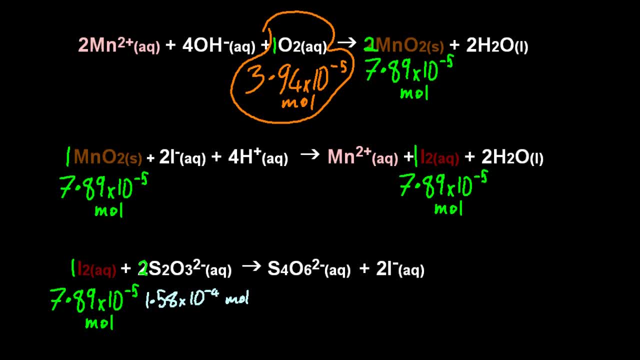 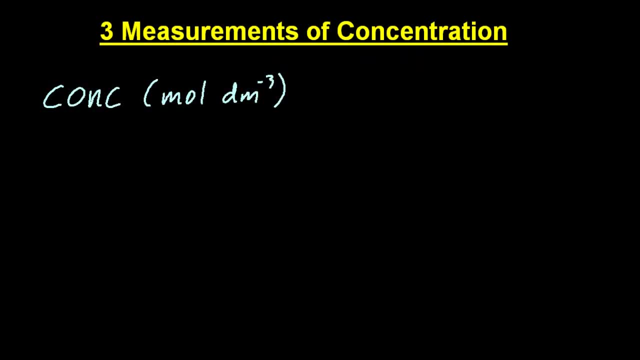 it. So that's the moles of oxygen dissolved in the water. There are three ways to measure concentration, So let's do all three three. So concentration in moles per decimetres cubed. Well, I just worked out the moles and the volume of water was 263 millilitres converted to decimetres. 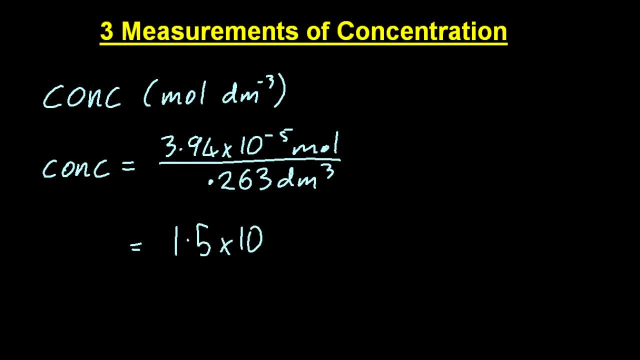 cubed. So that's the concentration in moles per decimetres cubed, Two sig figs. If I want to measure it in grams per decimetres cubed, concentration is going to be mass of the solute over the volume. the solution Now to work out the 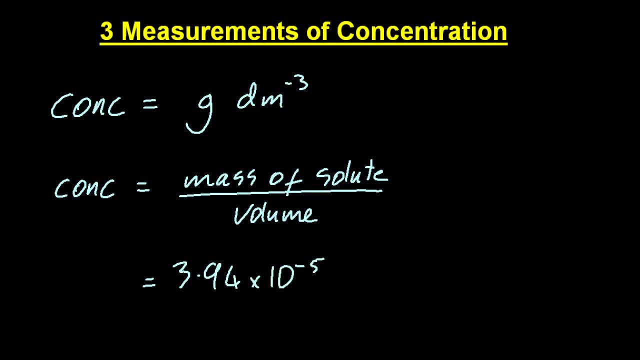 mass from the moles, you have to multiply by the molar mass of oxygen, which is 32 grams per mole, divided by the volume in decimetres cubed, and so my concentration is 4.8 times 10 to the minus 3 grams per decimetres cubed. 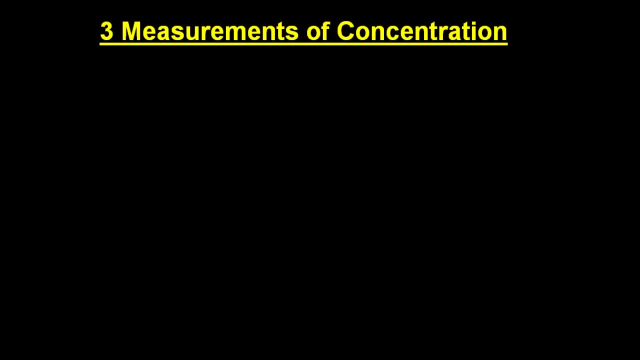 And in the question it asked in parts, per million. So that's the mass of the constituent, in this case oxygen, divided by the mass of everything. you've got times by a million. So the mass of the constituent, the oxygen. well, I know the. 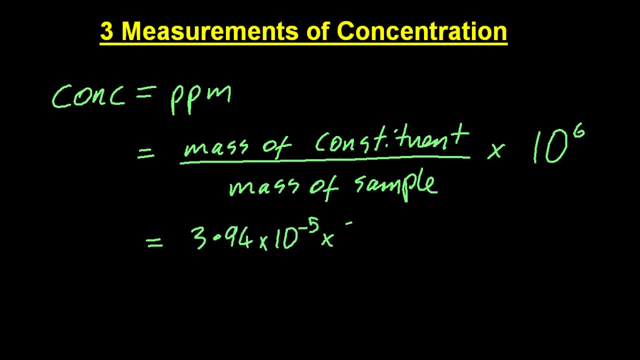 moles from my calculation before, multiplied by the molar mass gives me the mass of oxygen. And what's the mass of 263 millilitres? Well, I'm going to assume it's 263 grams. One millilitre of water is almost exactly one gram. It's not pure. 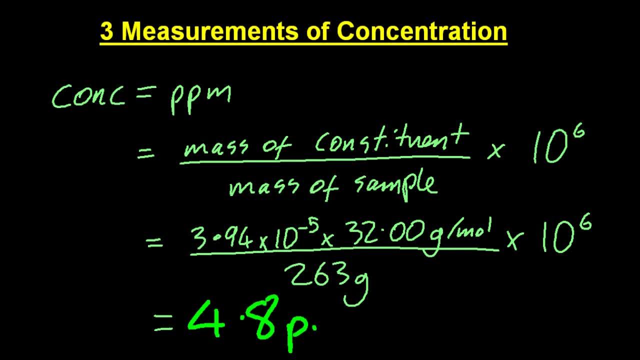 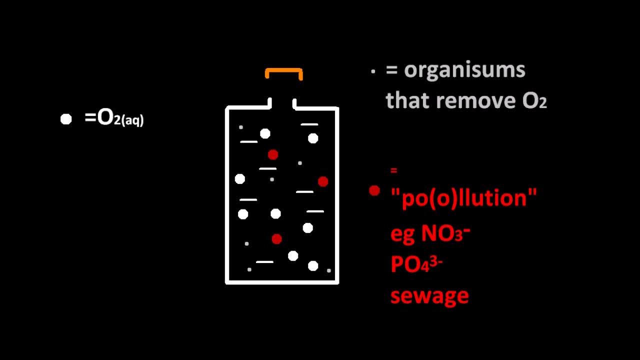 water, of course, Times by a million to give me 4.8 parts per million. So what about biological oxygen demand then? Well, get your sample of water, which probably has some pollution and some bacteria and organisms in it, Saturate it with oxygen, bubble oxygen through it until it will take no more oxygen Then.